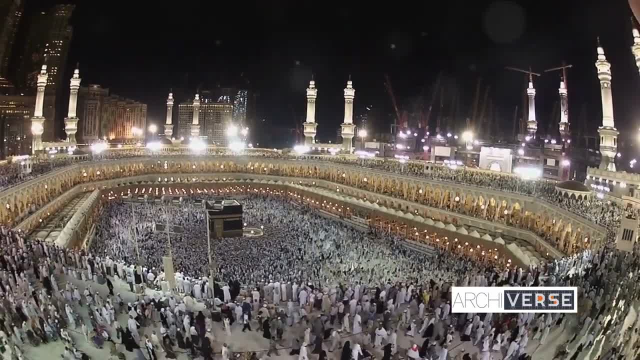 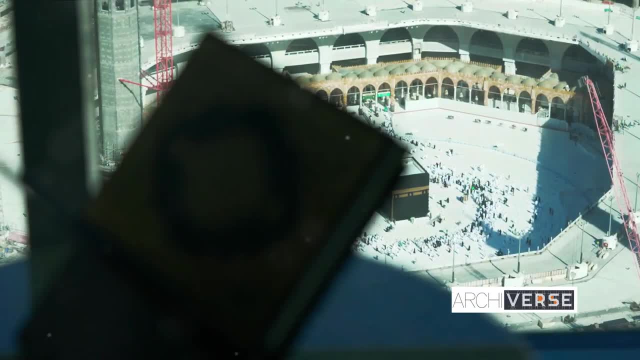 centuries. The structure we see today is a result of numerous transformations, each a testament to the evolving architectural prowess and the unyielding faith of its followers. Initially, it was a simple, unadorned cube of stones. Over time, it was transformed into a large 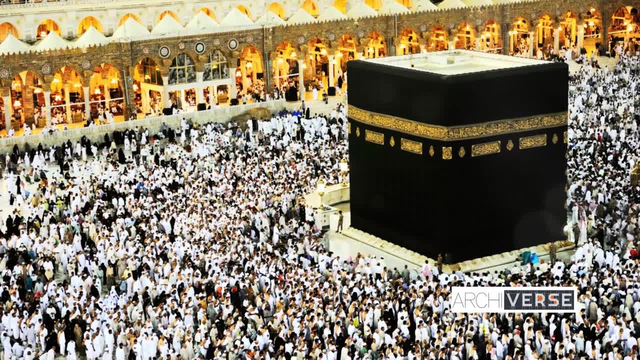 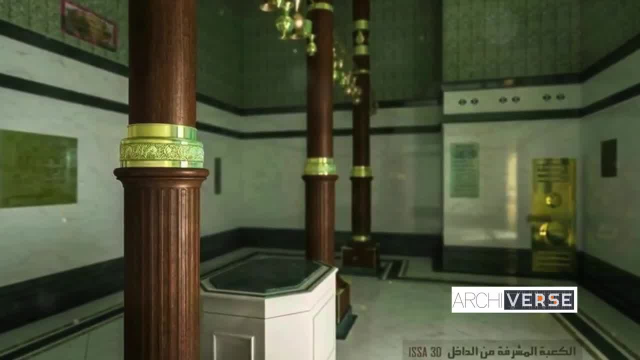 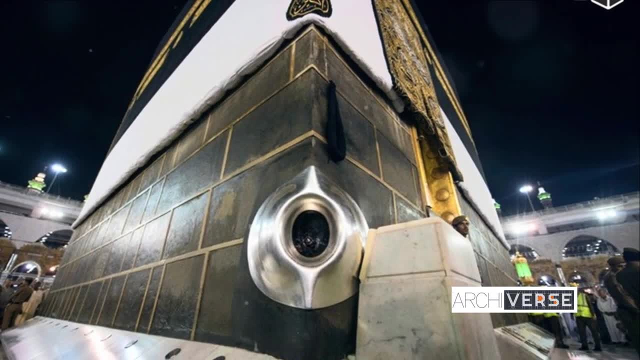 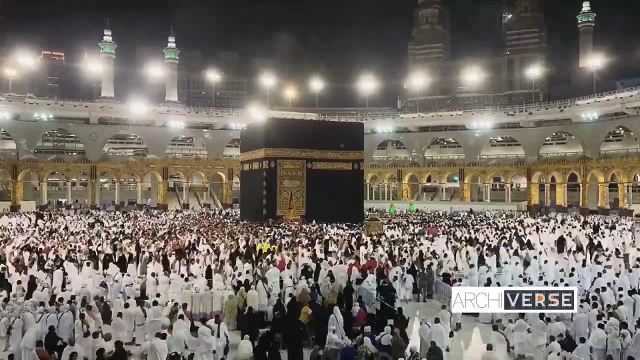 unadorned cube of stones. The Kaaba's interior, though rarely seen, is equally impressive, with marble and limestone walls. The structure also houses the sacred black stone believed to have been sent down from heaven. Despite its various iterations, the Kaaba's essence remains unchanged. 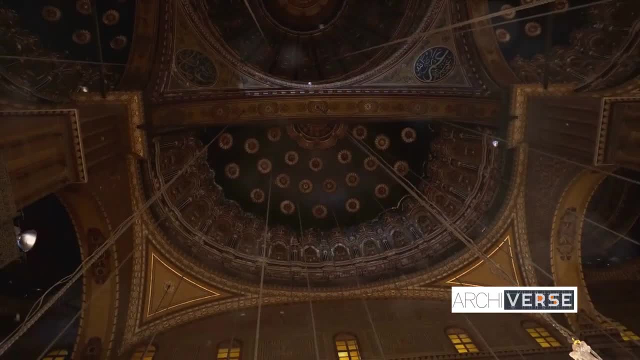 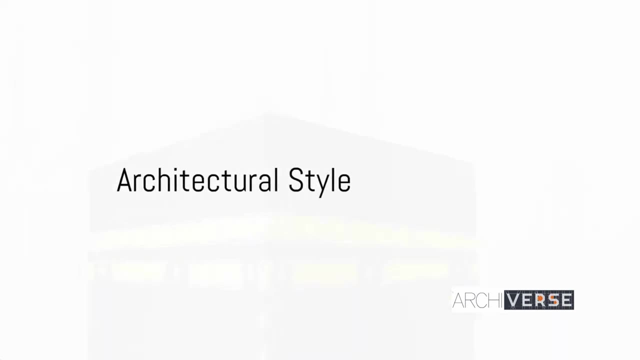 a symbol of unity, drawing Muslims worldwide towards it. The Kaaba's construction story is a testament to the unyielding faith and devotion of its followers. The Kaaba's architectural style is both simple and powerful. embodying the principles of Islamic architecture. Its cube-shaped. 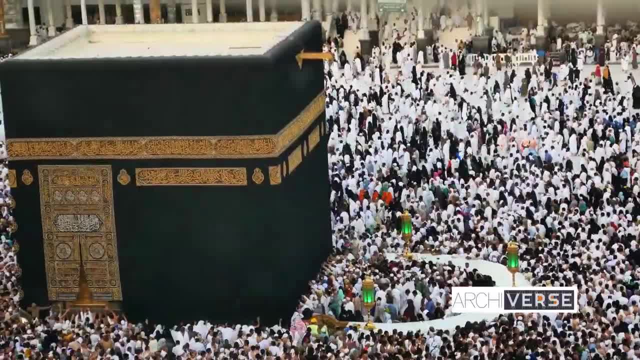 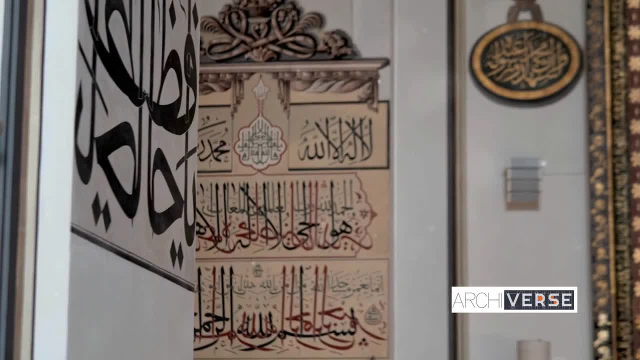 form, a geometrical shape known for its simplicity and strength, serves as a potent symbol of unity and purity, resonating with the Islamic belief in the oneness of God. But the Kaaba isn't just about simplicity. Its exterior, adorned with intricate calligraphy, showcases the beauty. 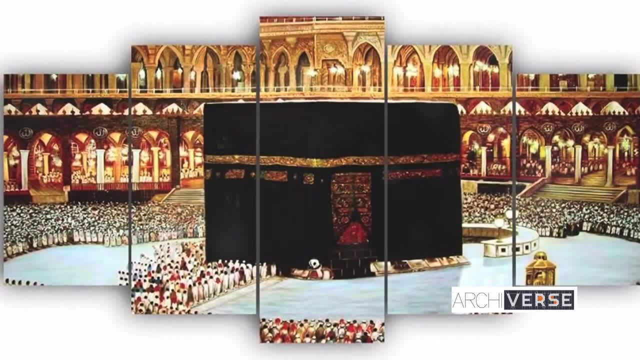 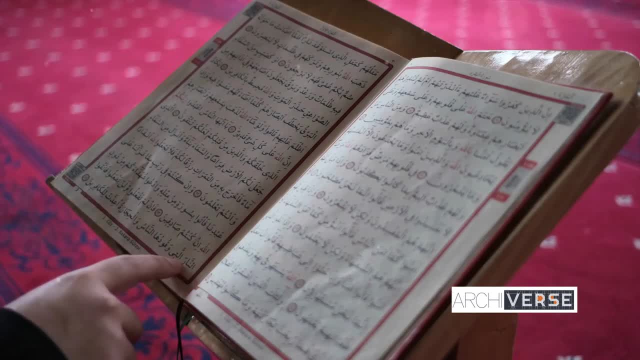 of Arabic script, a revered art form in Islamic culture. This calligraphy, woven into thefabric of the black silk covering known as the Kizwa, features verses from the Qur'an, the Holy Book of Islam. The combination of the Kaaba's simple form. 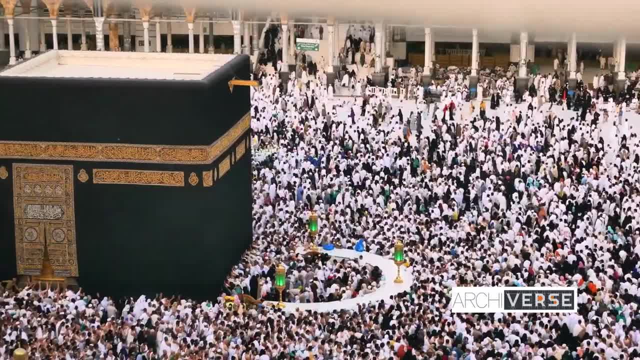 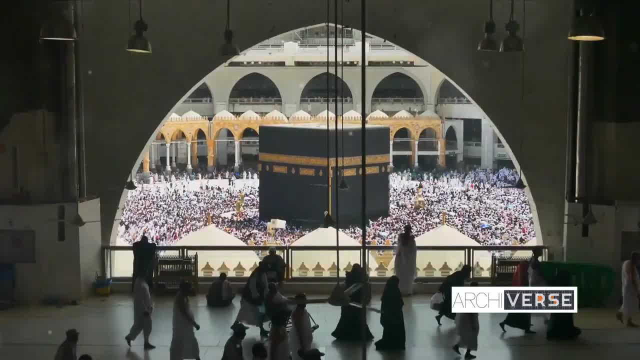 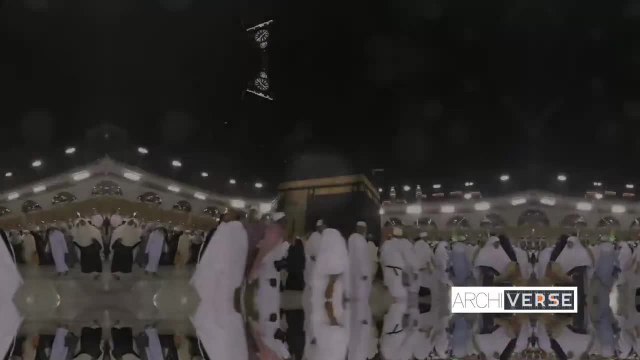 and intricate adornments creates a striking contrast reflecting the balance between simplicity and complexity in Islamic art and architecture. Despite its simplicity, the Kaaba stands as a timeless symbol of faith and devotion, a testament to the enduring power and beauty of Islamic architecture. 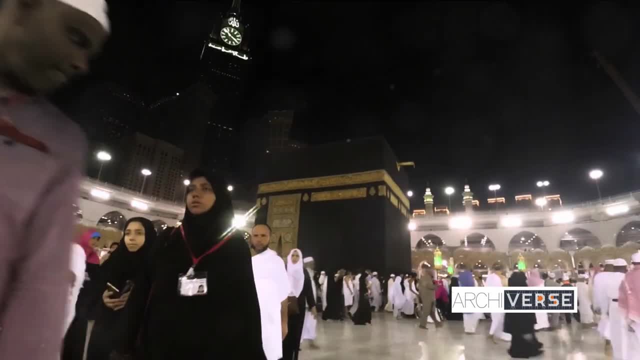 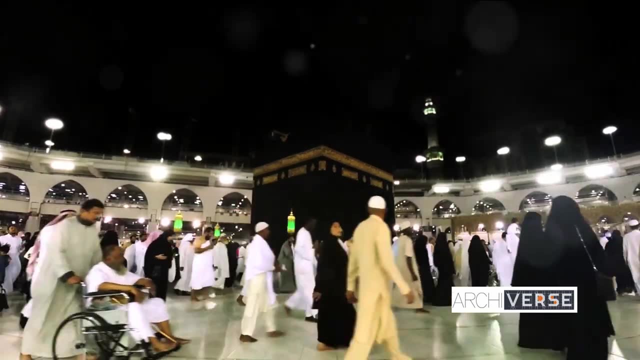 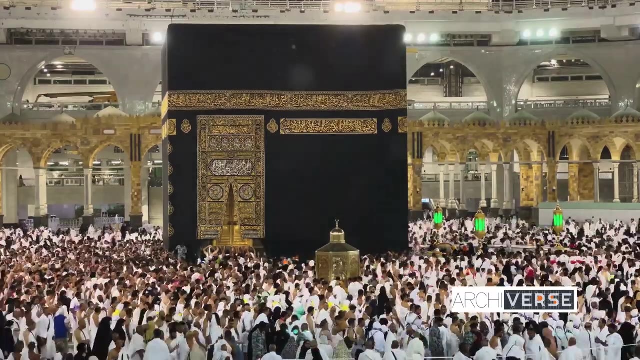 of the Kaaba's design holds deep symbolism and meaning. To start, let's consider the sacred black stone Set into the eastern corner of the Kaaba. it is believed to have descended from heaven. This revered relic draws millions of Muslims who strive to kiss or touch it during the Hajj pilgrimage. 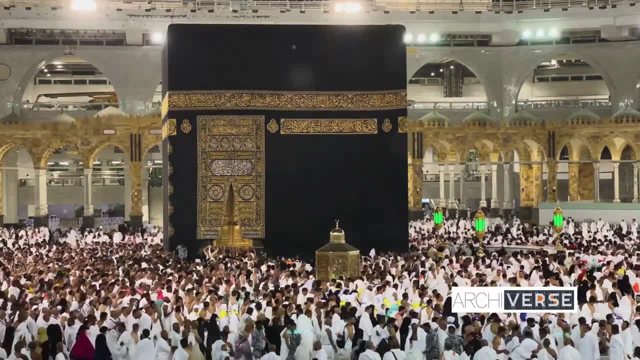 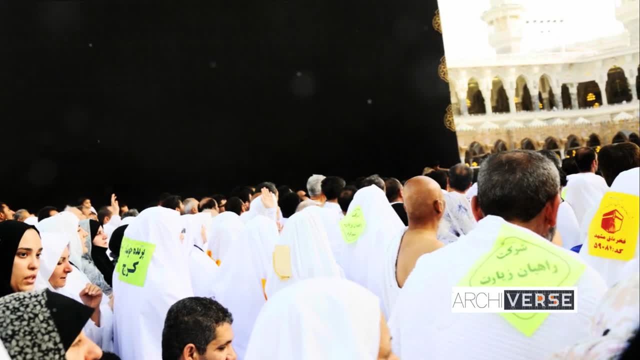 a practice traced back to Prophet Muhammad himself. Next, the golden door, located close to the ground on the northeastern wall of the Kaaba, is another significant design element. It is not just a door, but a gateway to a space holding immense spiritual value for Muslims worldwide. 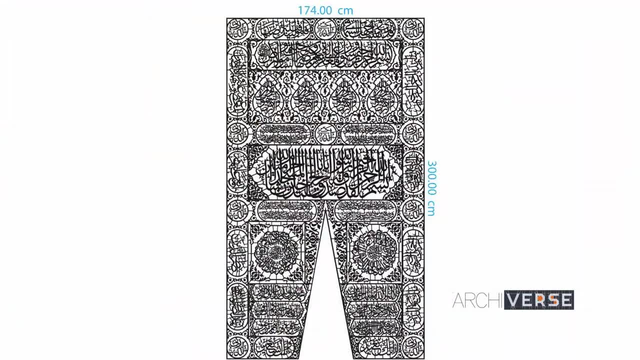 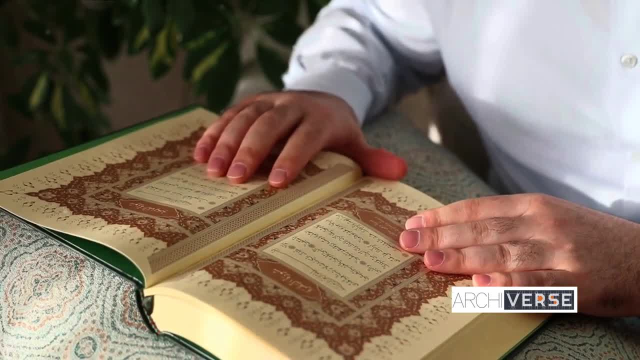 Finally, let's talk about the Kiswah, the black silk covering that drapes the Kaaba Embroidered with verses from the Quran. in gold and silver threads it is replaced annually during the Hajj season, symbolizing renewal and continuous devotion. 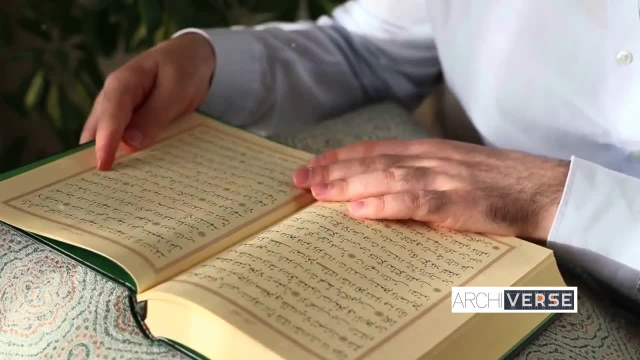 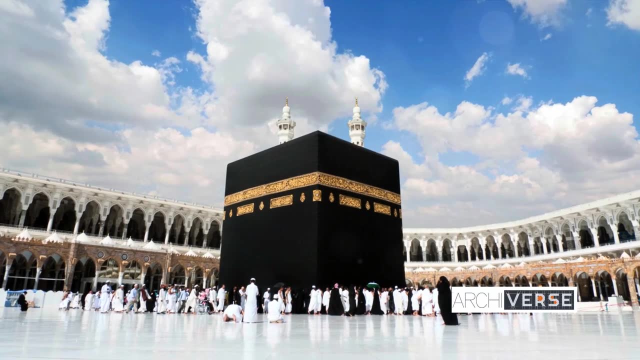 The Kaaba's design is a testament to the rich cultural heritage of Islam. Did you know that the Kaaba is the only religious structure in Islam that does not have any idols or images inside? That's right, this cube-shaped building sitting at the heart of Mecca. 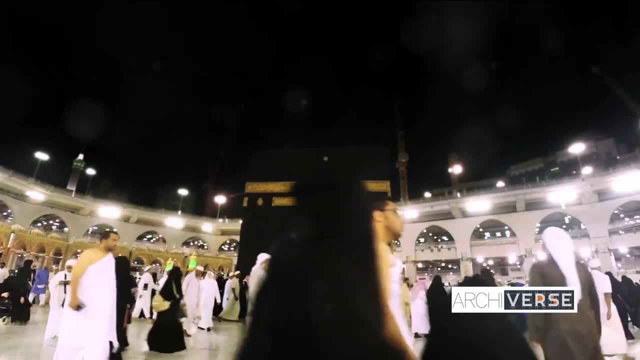 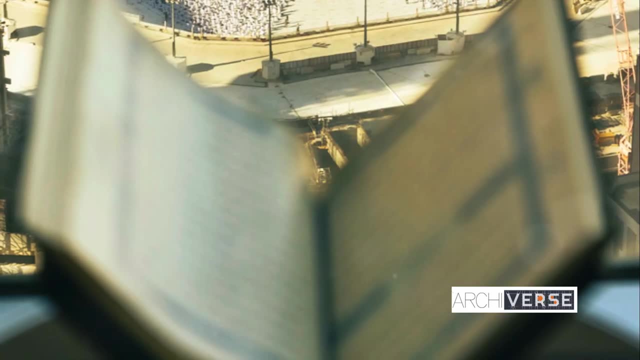 is void of any interior decorations or religious symbols. Instead, the interior is a simple, unadorned space, further emphasizing the Islamic principle of monotheism. Now let's move to its exterior. You might be surprised to learn that the Kaaba's black silk covering 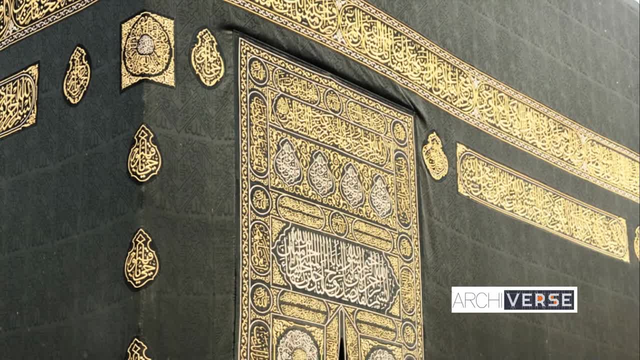 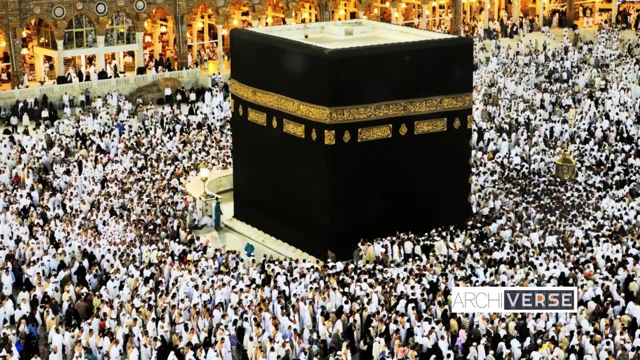 known as the Kiswah, is replaced annually during the Hajj pilgrimage. The Kiswah is made in a special factory in Mecca and is embroidered with gold and silver threads bearing Quranic verses. Ever wondered about the Kaaba's dimensions? 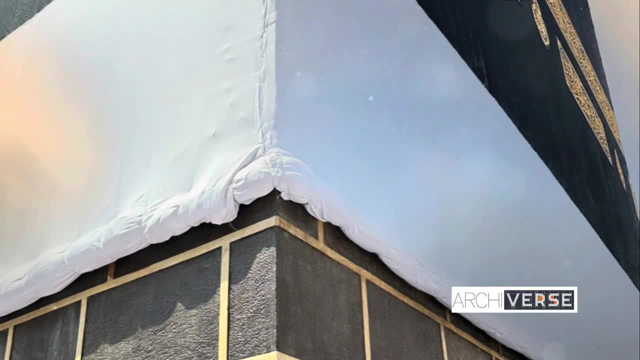 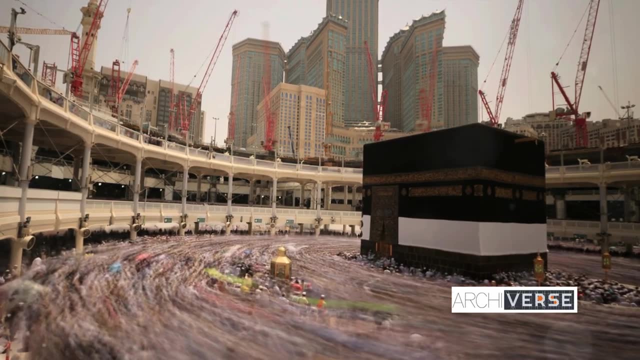 The Kaaba stands approximately 43 feet high and its walls are about 7 feet thick. Despite its grand appearance, the Kaaba maintains a humble, cube-like shape, hence its name, which means cube in Arabic. The Kaaba is also known as the House of Allah. 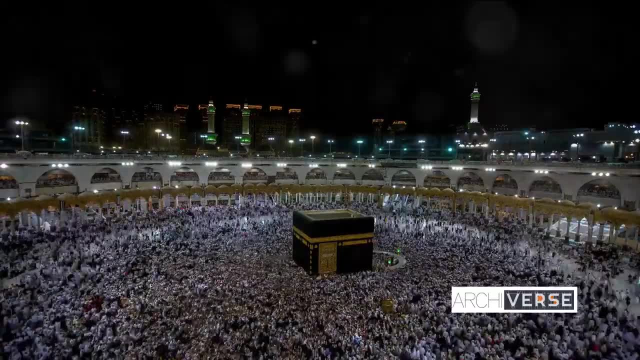 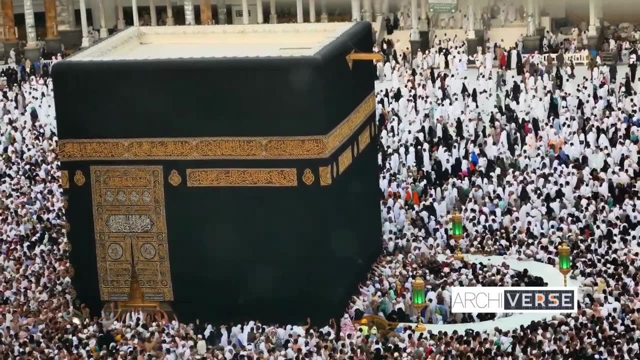 It's the point towards which all Muslims around the world direct their prayers, no matter where they are located. This unified direction of prayer, or Qibla, symbolizes the unity and equality of all Muslims. Finally, here's a fact that might astonish you. 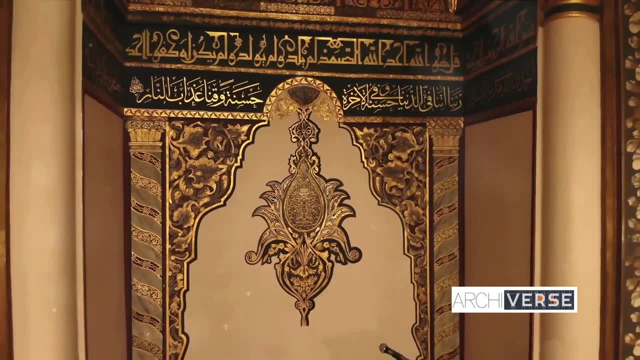 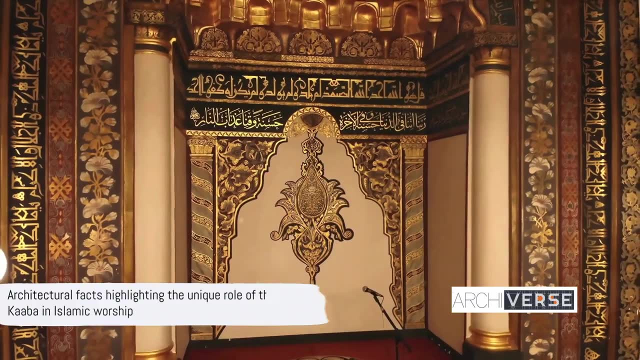 The Kaaba has been reconstructed multiple times over the centuries, the last major rebuild happening in the early 14th century. These architectural facts further underline the Kaaba's unique role in Islamic worship. As our journey comes to an end, we can only marvel at the timeless beauty. 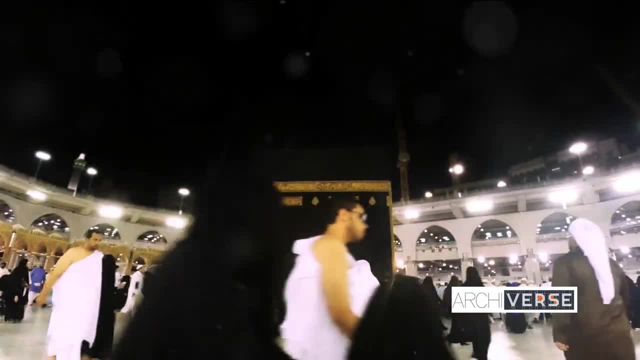 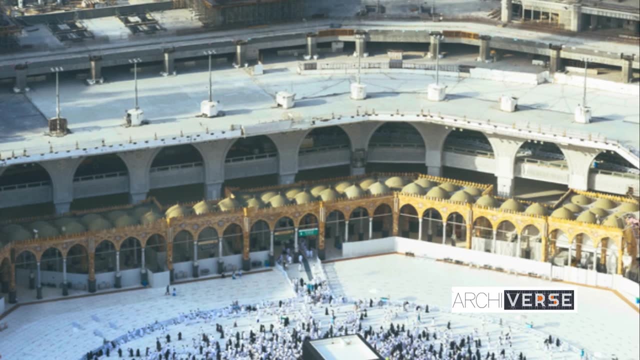 and spiritual significance of the Kaaba. This architectural marvel is not merely a physical structure. It is a symbol of faith, unity and devotion for millions of Muslims worldwide, From its humble beginnings as a cube-shaped structure in the heart of Mecca. 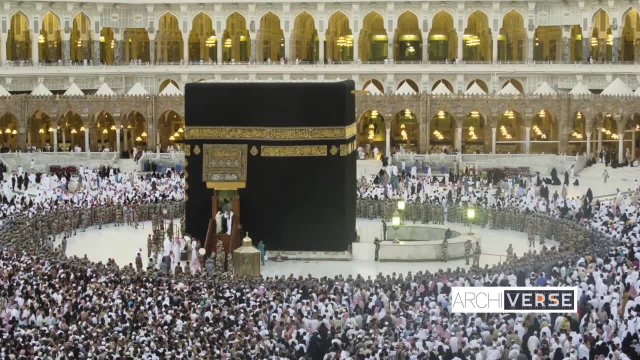 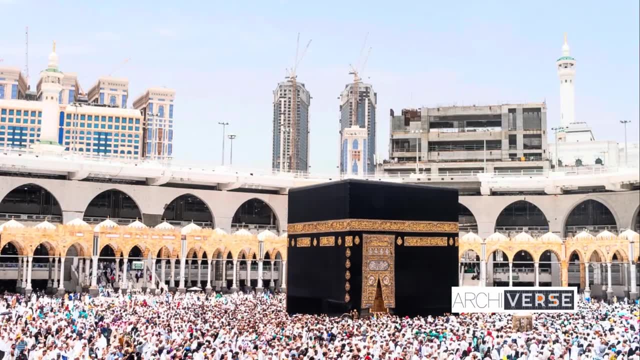 to the grandeur it embodies today. the Kaaba's history is steeped in rich cultural heritage. Its construction details, architectural style and design elements all tell a story of devotion and unity that spans centuries. The Kaaba with its intricate calligraphy and symbolic design elements.